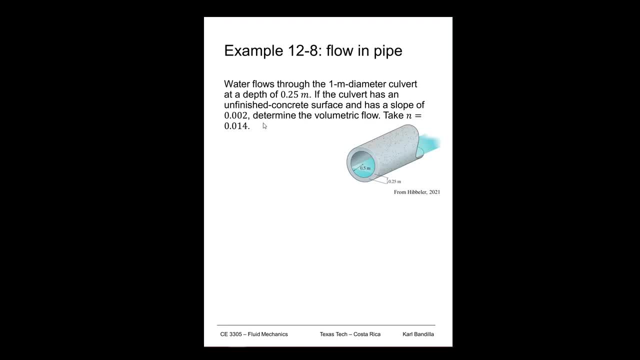 concrete surface and a slope of 0.02.. We want to get the flow rate and we're given what the surface roughness coefficient is. All right, so what do we do? Well, we know we have a formula that will give us our area and our wetted perimeter, but it depends on kind of this. 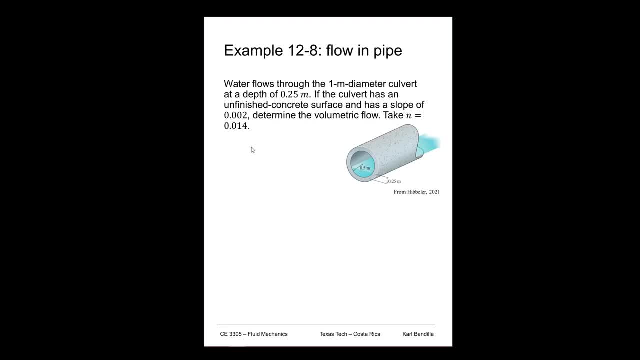 angle right. So we'll have to figure out what that looks like. So if we draw our cross section somewhat of a circle here, like this, Let's choose a different color. All right, we know that we have our depth here. All right, we know that this distance, we'll call that distance, we'll call it. 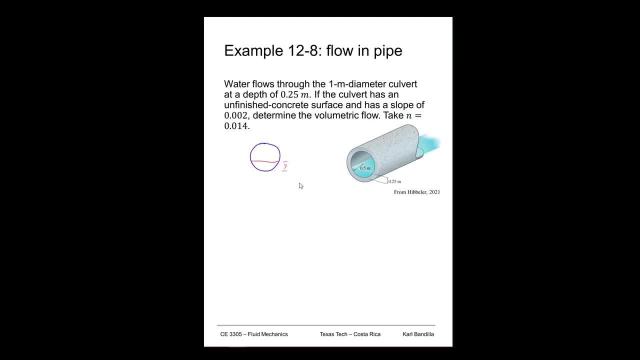 y, Let's do it, Do an arrow here. All right, this would be our depth y. We know that we have a center somewhere, So we know that this whole distance here is, of course, the radius. We know that this is also the radius. All right, so if this is the radius and this lower, 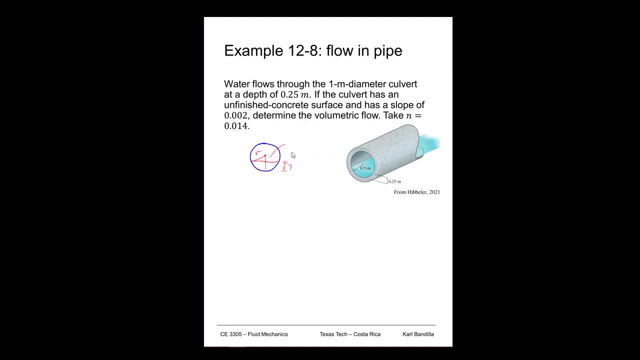 part is y, then we know that we're going to draw this somewhere else. here have some space, right. So we know that this here, that little piece right there, that piece in green light- green doesn't show up all that well. All right, we know that this. 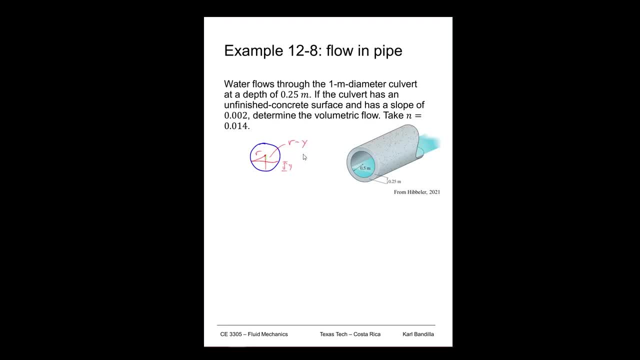 place would just be r minus y, And the angle that we're interested in is the little angle in here right, And we'll call that angle theta, All right. so how do we get that angle? Well, we'll have a nice triangle here, right? We don't know what this part of the triangle? 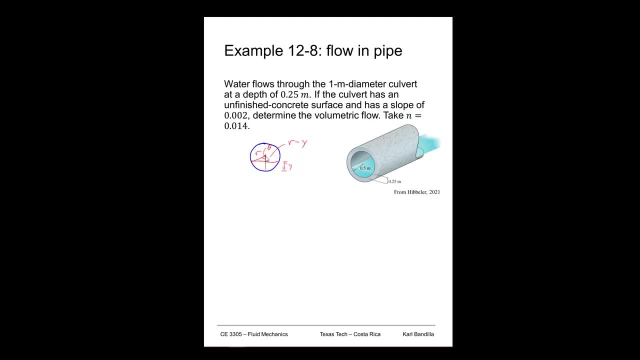 but we know the hypotenuse is and we know what the adjacent leg is right. So we can say the cosine of theta is going to be r minus y, which is that little piece that I colored in green, divided by the hypotenuse, which is r. Okay, so we're trying to find the angle. So let's say: 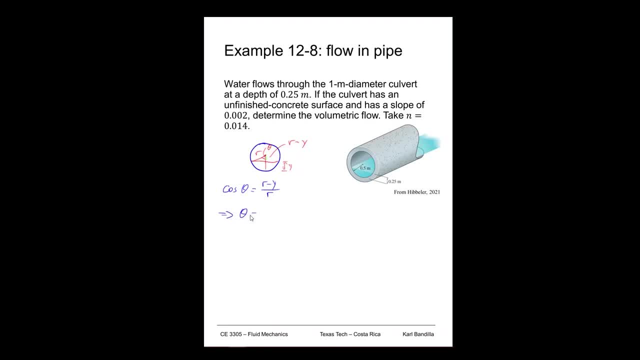 that means that theta is, of course, cosine minus one over that term, r minus y divided by r, which is, we put in numbers, cosine minus one of 0.5 meters minus 0.25 meters divided by 0.5. 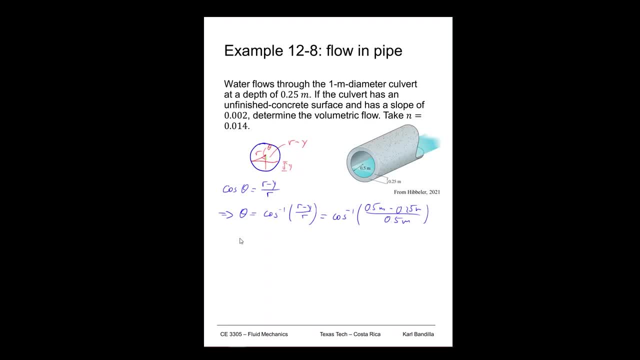 meters, And that is equal to cosine minus one of 0.5.. And now, very importantly, we're doing all this in radians right, Not in degrees. But if we know the cosine right, then we know that this is pi over. 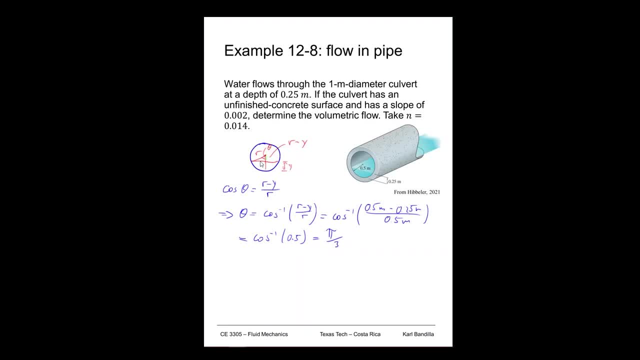 three. Now we're not interested in that half angle, we're interested in the full angle. So my alpha, that is going into all my equations, is going to be two times theta. So that would be two pi over three. right, That's our. 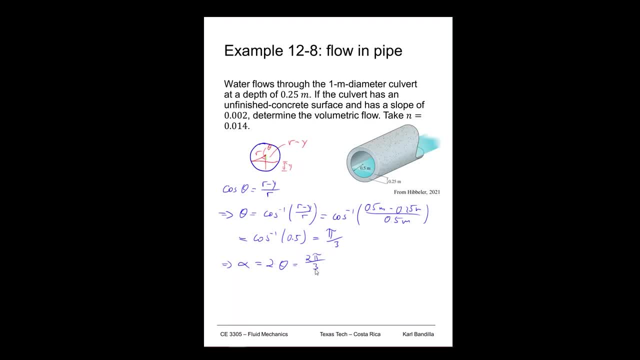 opening angle. that goes into into our two equations that we have, one for the flow area, the other one for the wetted perimeter. So we start with the area. then we can say a is equal to r squared over two times alpha. time not times, but minus sine alpha. This is why we have to have our angle in radians, right. 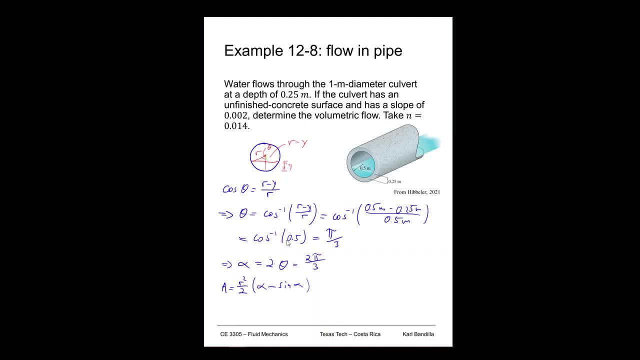 For the sine it doesn't matter, but up here it has to be in radians, All right. so let's plug it in, So that'd be 0.5 meters for our radius, squared right at a, at a one meter diameter, divided by: 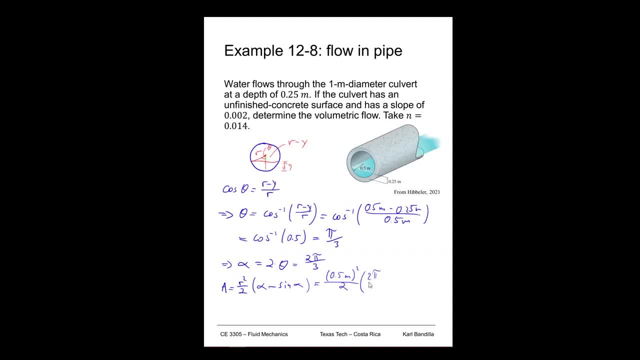 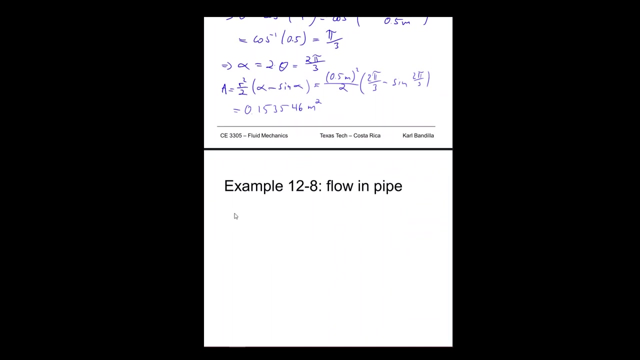 two and then times 2pi over three, minus sin of two pi over three, And that is equal to 0.153546 meter squared, And that's our flow area. Now we also need to have our wetted perimeter, So that equations 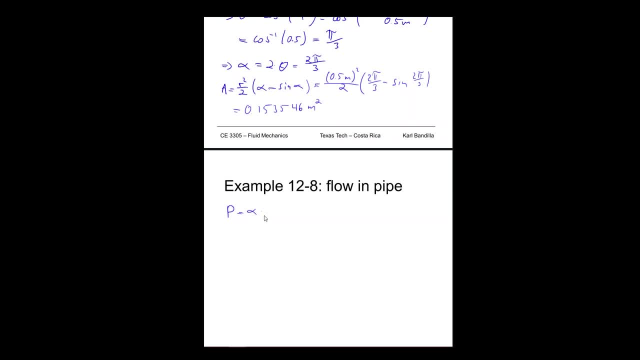 even easier. P is equal to alpha times R, So for us 2 pi over 3 times 0.5 meters, So that is 1.047198 meters. Alright, with that we can get our Q. Q is equal to A to the 5. 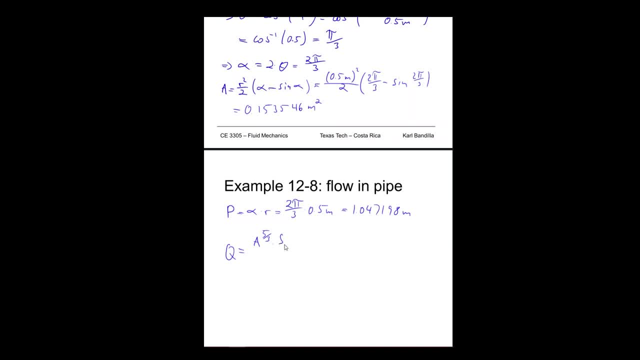 thirds times the slope square root of the slope, divided by N, which is the unknown, without an exponent, and then P to the 2 thirds. Alright, so that is 0.153546 meters squared to the 5 thirds Times. the slope was 0.002, times 0.002 to the 1 half square root. N is given to us. 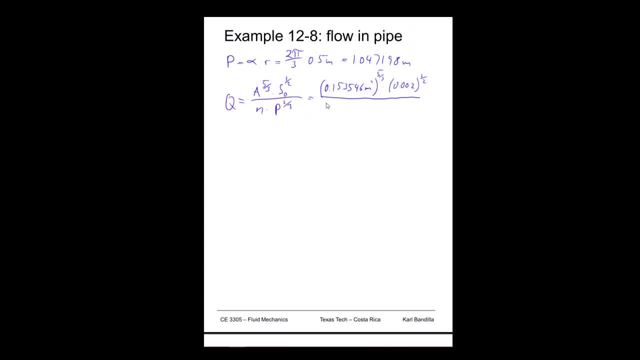 as 14,, so 0.014,, and then again our strained unit S over meters to the 1 third Times. and then our, our wetted perimeter, 1.047198 meters to 2 thirds. Alright, so that. 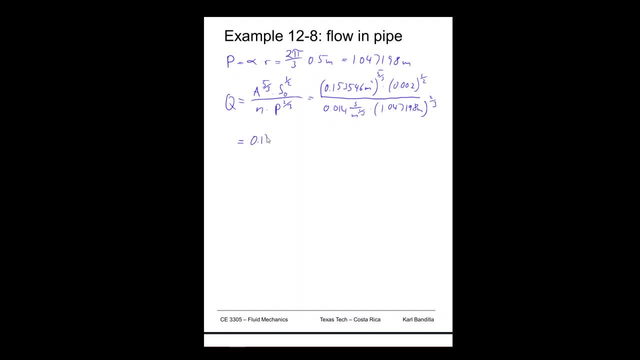 is then 0.136385 cubic meters per second. Alright, so that is then 0.136385 cubic meters per second. Alright, so that is then 0.136385 cubic meters per second. Let's see if that makes sense. Where are our seconds are right here, so that is good. 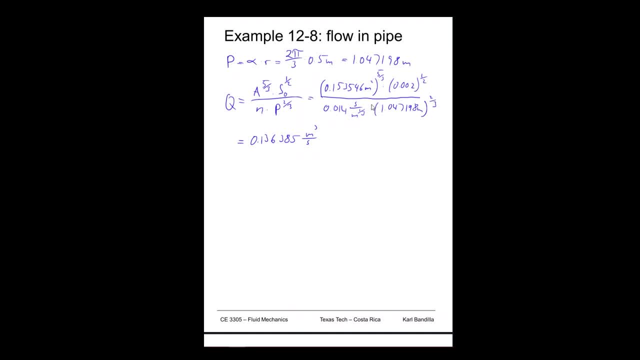 Now our meters. What do we get? We get up here. we get 10 thirds. Let's do down here for 10 thirds plus 1 third will be 11 thirds. Let's do a little 11 up here, So it will be.